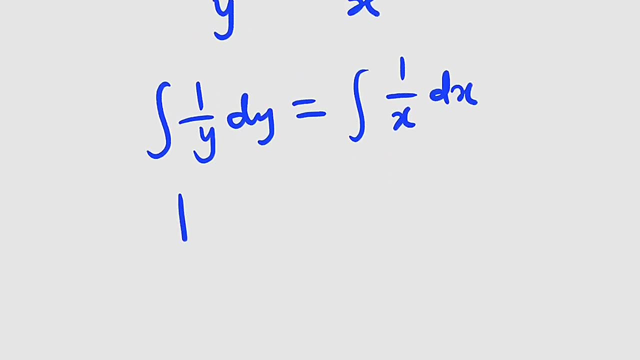 If you integrate 1 over y, you're going to obtain natural log of what absolute value of y. If you integrate 1 over y, you're going to obtain natural log of what absolute value of y. If you integrate 1 divided by x, the same thing: natural log of the absolute value of x. 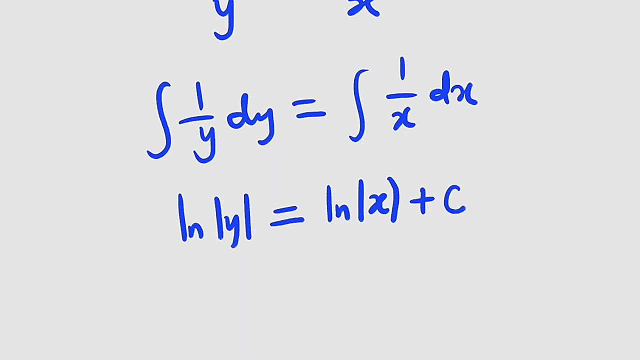 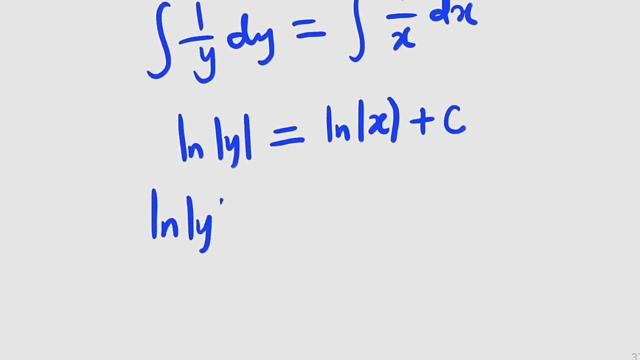 But remember the constant of integration. But a constant is the same thing as natural log of a constant right. So we can write this as natural log of absolute value of y, equal to natural log of the absolute value of x plus natural log of c, By applying one of the laws of logarithm. 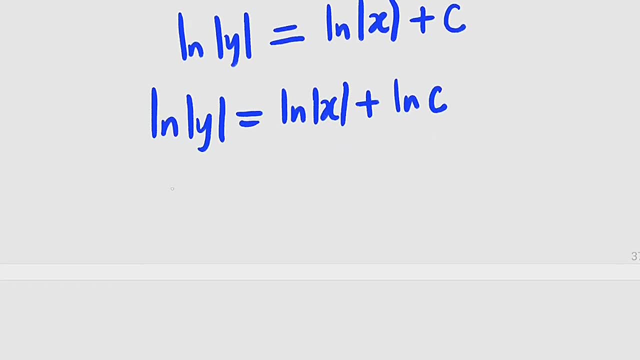 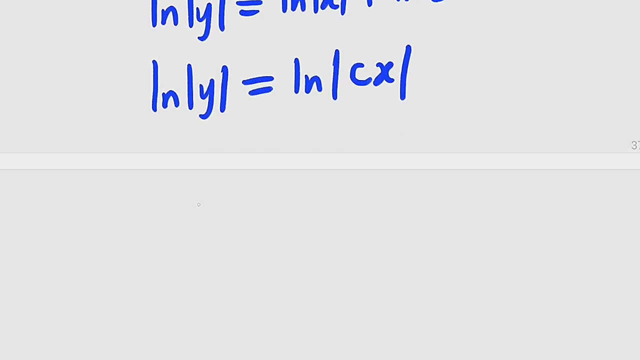 you can assign this a single log. So the left hand side: we have natural log of what absolute value of y and this is equal to natural log of absolute value of cx. Both sides we have natural log which implies that y is equal to cx. Final answer: Here is another one. 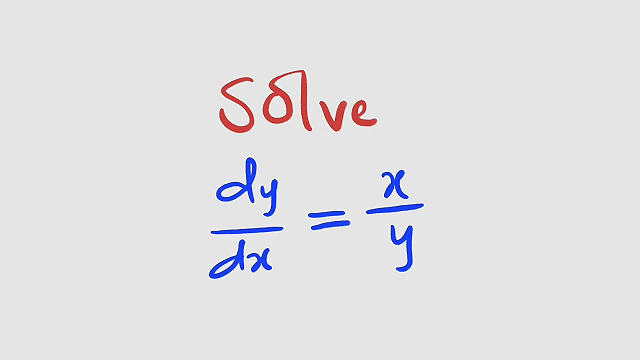 We are given that dy over dx is equal to x divided by 1. divided by x- x. Here we gotta know that they mean that dx equal to x. suppose that i look at my y give x equal to x over x by x squared. so here's the previous work. how many times did i say all these numbers? 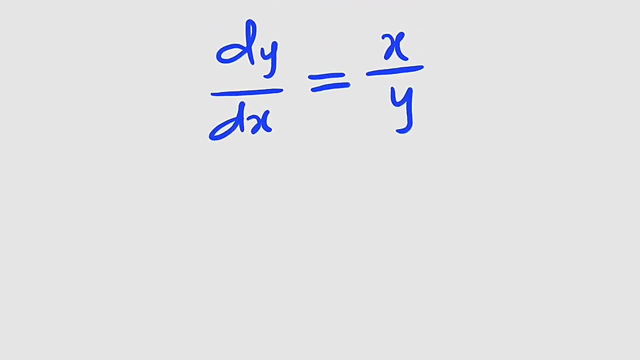 by y. by applying variable, sub variable, we're going to bring y to the left hand side and take dx to the right hand side. by cross multiplication we have y, dy equal to x, dx. integrate both sides, integrate this. you have to integrate this to the left hand side. we are going to have 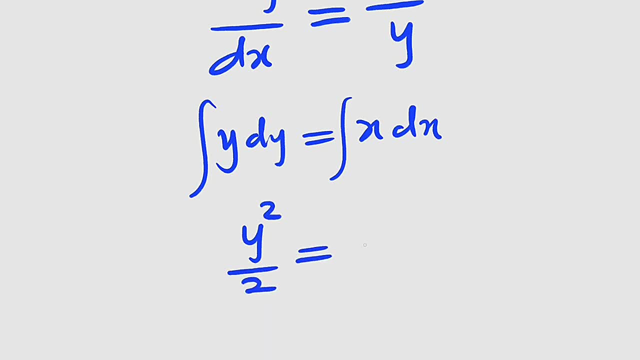 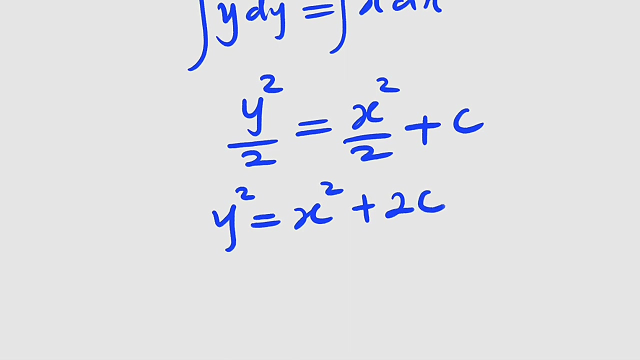 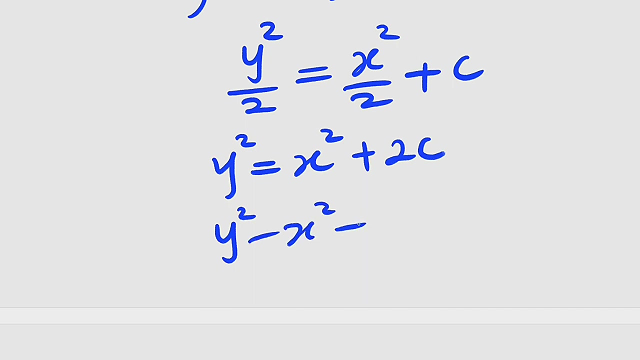 y squared divided by 2. to the right hand side, we have x squared divided by 2, plus the constant of integration. multiply both sides by 2, y squared equal to x squared plus 2c. you can take x squared to the left hand side if you like. so we have y squared minus x squared equal to 2c, which i can. 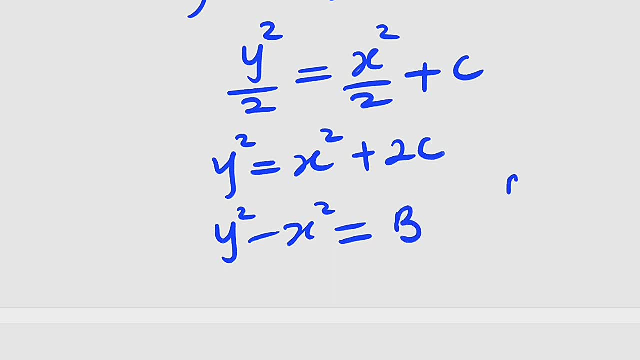 write as, let me say, b, for which b is equal to 2c. they are all constants and this is just the solution to this problem. thank you for watching, do share to your learning colleagues and don't forget to subscribe to my youtube channel for more exciting videos. bye.